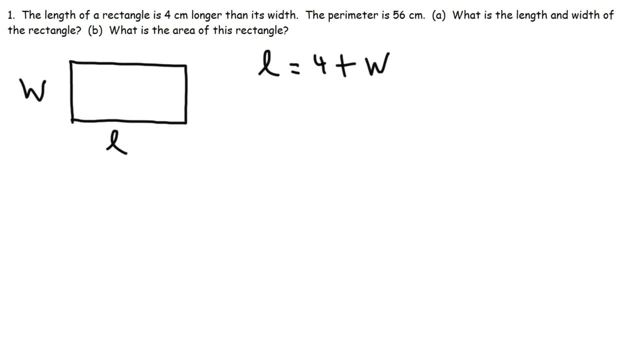 If you have three variables, you need three equations to solve it. The other equation is the perimeter equation. Perimeter is equal to 2L plus 2W. The perimeter is the distance around the rectangle. So keep in mind we have L here and W here. 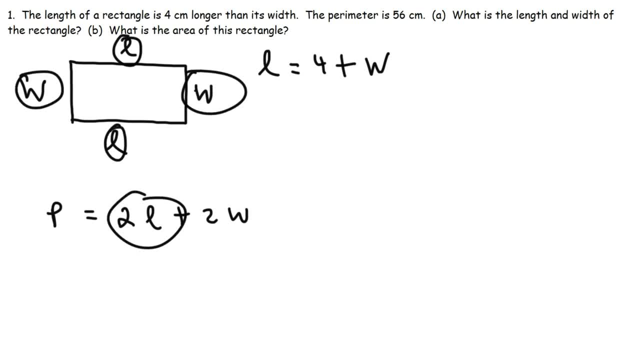 So L plus L gives us 2L. W plus W gives us 2W. Now what we're going to do is we're going to replace P with 56. So we have: 56 is equal to 2L plus 2W. 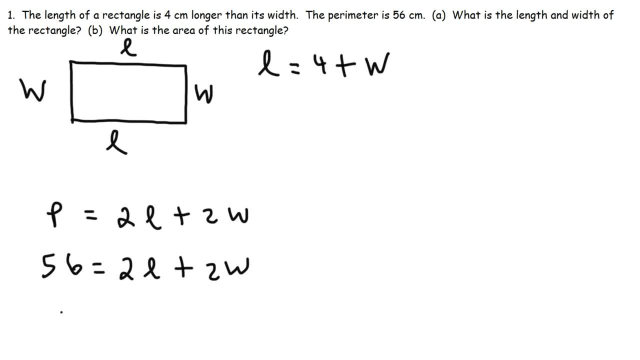 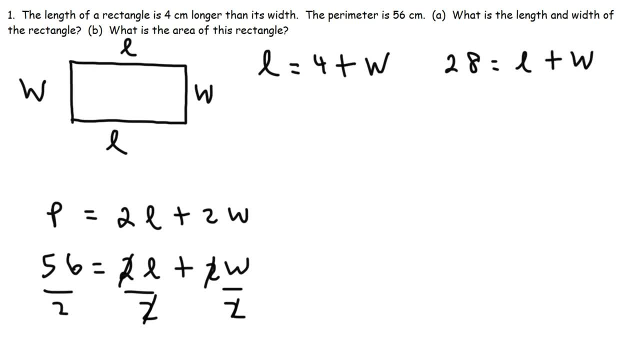 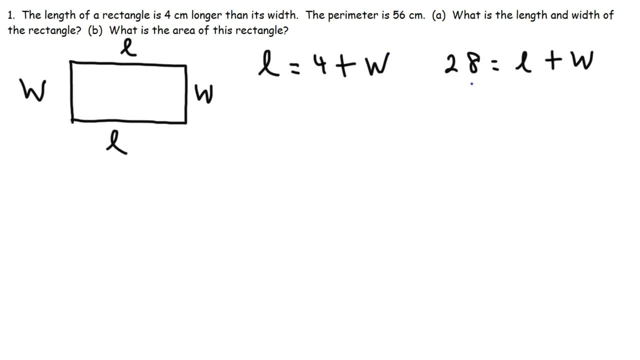 So we're going to solve this system by substitution. We're going to substitute L with 4 plus W, because L is equal to 4 plus W, So let's go ahead and do that. So this is going to be 28.. And then, instead of writing L, we're going to write 4 plus W. 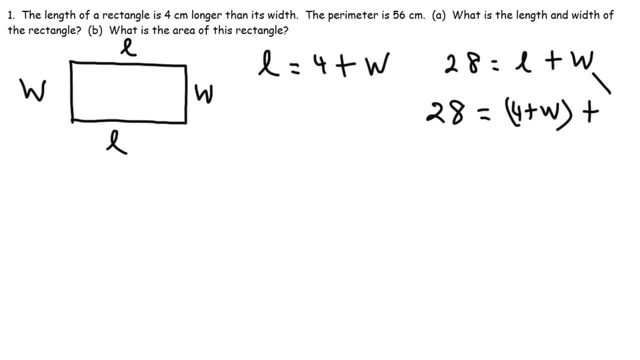 So that was L, And then plus the other W that we have here, W plus W gives us 2W. So at this point we have 2W And we have one equation and one variable. So now we could solve for W. 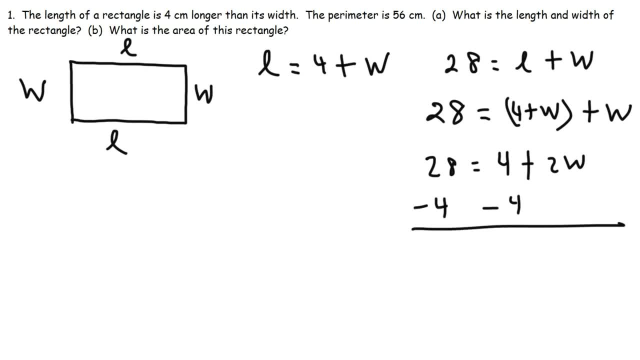 Let's subtract both sides by 4.. 28 minus 4 is 24.. And we could bring down the 2W, So 24 is equal to 2W. Next, we could divide both sides by 2.. 24 divided by 2 is 12.. 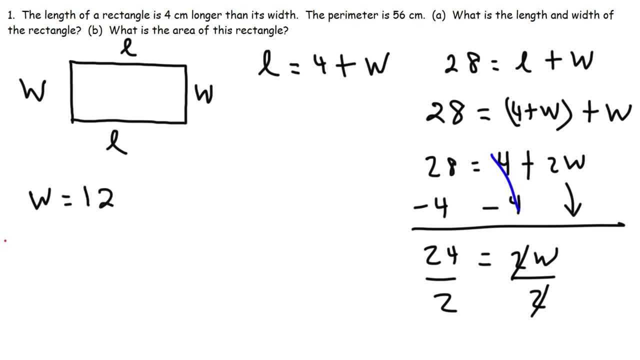 So we get that W is 12.. And the unit, The unit, The units are centimeters. So W is 12 centimeters. So that is the width of the rectangle. Now let's calculate the length, So we can plug in W into this equation. 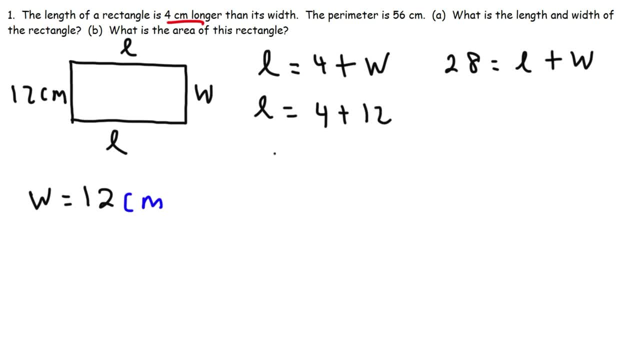 So L is going to be 4 plus W, or 4 plus 12, which is 16.. So now we have the width of the rectangle and the length. So that is how you can find the length and the width of the rectangle. 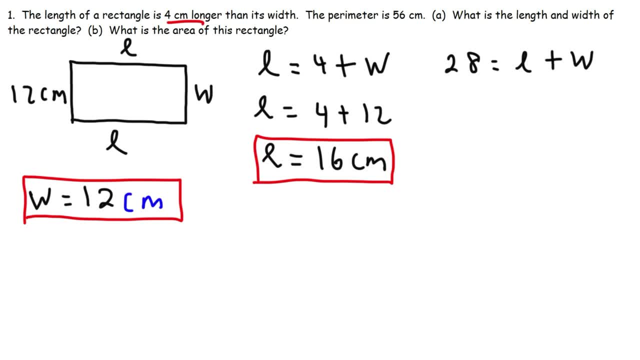 If you are given the perimeter Now, the last thing we need to do in this problem is calculate the area of the rectangle. The area of the rectangle is simply the product of the length and the width. So we have the length of 16 centimeters. 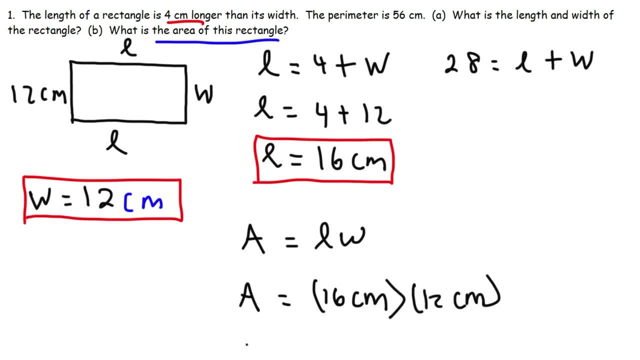 and the width of 12 centimeters. So we have to be able to get the length as well And the width of that clerk. to multiply those two numbers 16 times 12 is 192.. And then we have centimeters times centimeters. So you add the exponents and you'll get centimeters. 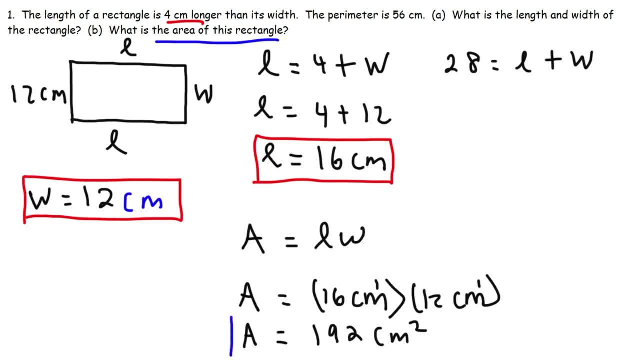 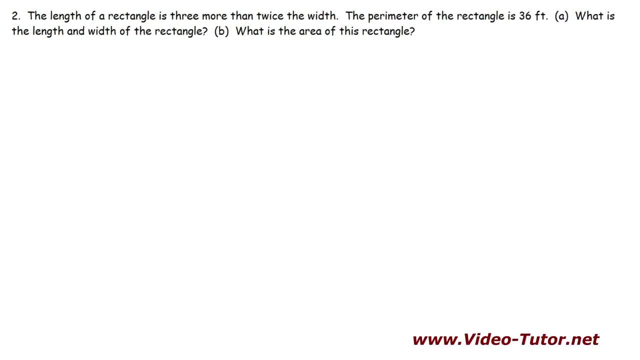 square. So that is the area of this particular rectangle. It's 192 square centimeters. Now let's work on another problem. It's similar, but slightly different. If you want to pause the video and try this example, feel free to go. 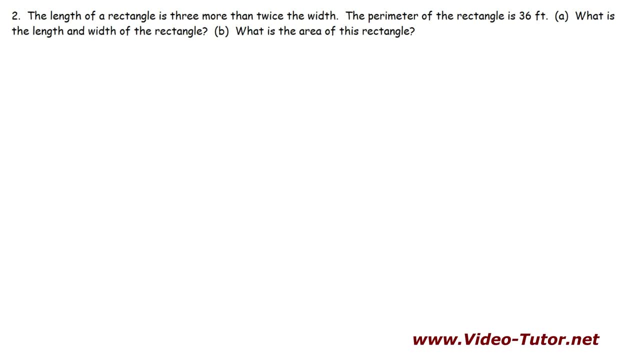 ahead and do that. Number two: the length of a rectangle is three more than twice the width. Now we're given the perimeter. The perimeter of this rectangle is 36 feet. What is the length and the width of the rectangle? So let's begin by drawing a. 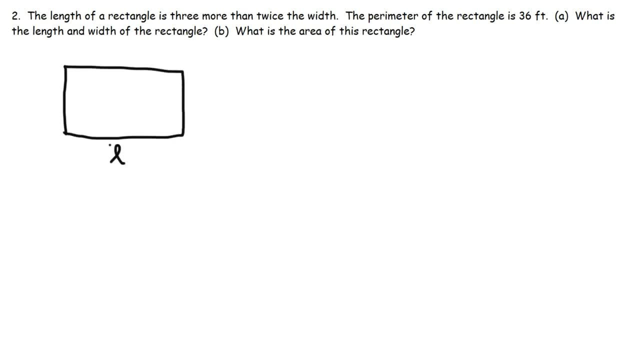 picture. So we have L and W. Now the first thing that we need to do is we need to write an equation that relates L and W. So we're told that the length of a rectangle is three more than twice the width of the rectangle, Three more than twice the 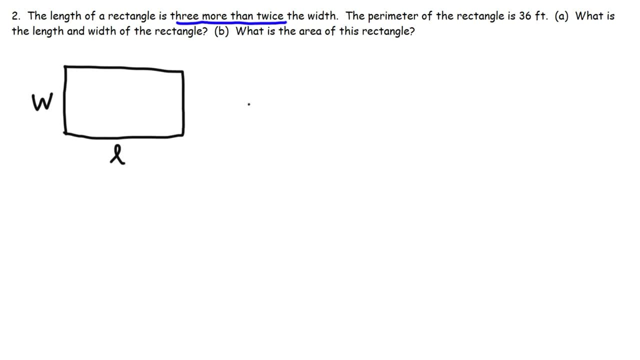 width. How can we represent that as an equation? So, if we read it from left to right, the length of the rectangle- so we're talking about L- is means equal. So we have three, three more, so three plus something. 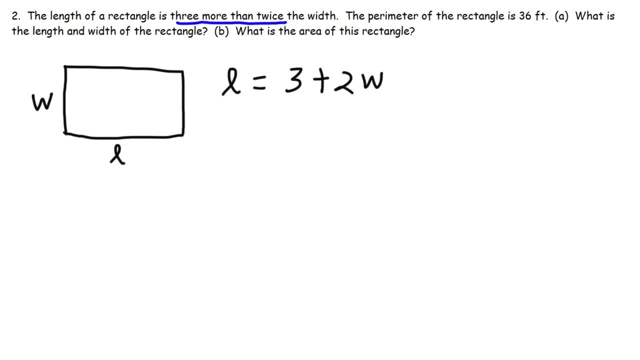 Then twice the width, so two times the width. Now we still have our other perimeter equation: p is equal to 2L plus 2W. The perimeter in this example is 36 feet. Now, just like before, since everything is equal, going to try and create the second diamond. Now, just like before, since everything is equal, we need to. 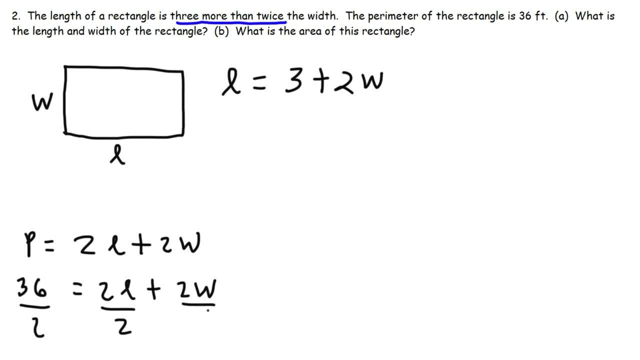 even we could divide each of these numbers by 2.. 36 divided by 2 is 18.. So we have: 18 is equal to L plus W. So at this point we have two equations and two variables. So now we could solve the. 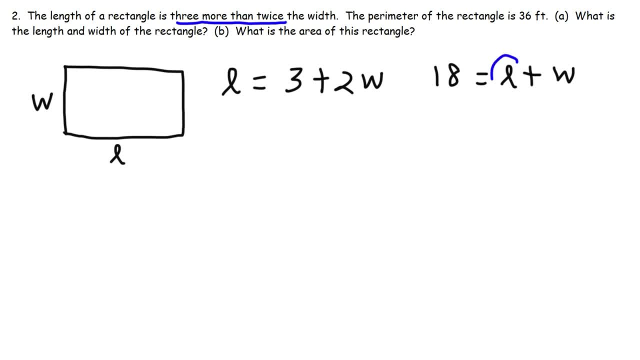 system of equations by substitution. Just like before, we're going to replace L with 3 plus 2W, since that is equal to L, So let's go ahead and plug it into the second equation. So we're going to have 18 is equal to. instead of L, we'll write 3 plus 2W and then plus the other W here. 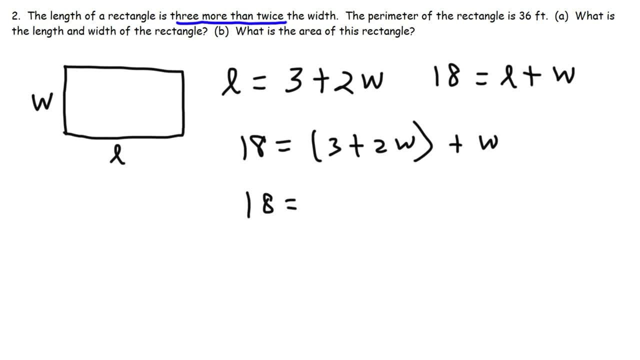 Now we can combine 2W and 3W And 1W. that will give us 3W, So we have 3 plus 3W. Now all of these numbers are divisible by 3.. So let's go ahead and divide these numbers by 3.. 18 divided by 3 is 6.. 3 divided by 3 is 1.. 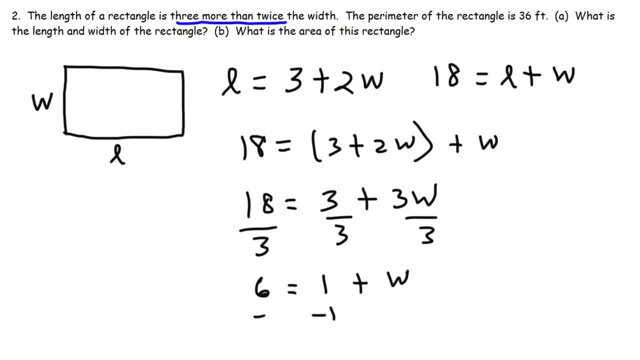 3W divided by 3 is just W. Next, we could subtract both sides by 1.. 6 minus 1 is 5.. So we get that W. The width of the rectangle is 5 and the unit will be in feet, So 5 feet. 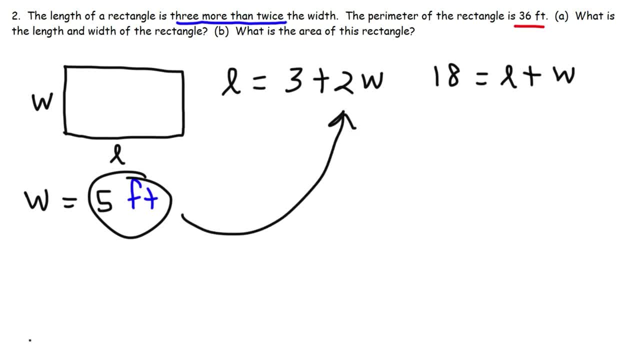 Now that we have W, let's go ahead and plug that in to get L. So L is 3 plus 2W. So let's replace W with 5.. 2 times 5 is 10.. And 10 plus 3 is 13..